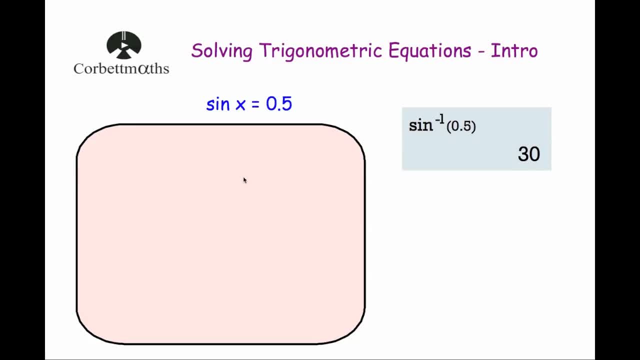 of 0.5 and you would get 30 degrees. Now if we look at the sine graph, you may notice that from the sine graph, whenever we look at 0.5 here, 30 degrees wouldn't be the only solution. You can see 30 degrees would be a solution, but then there's 0.5.. So if we 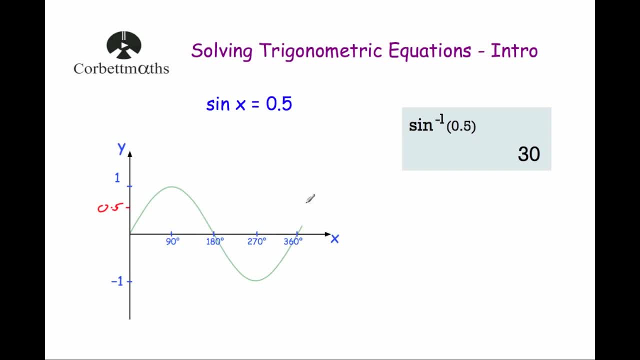 look at the sine graph, there's another solution over here and actually if we carried on the graph there'd be more solutions as we go along. So whenever we're solving trigonometric equations, we've got to be quite careful whenever we get our answers, because there won't just 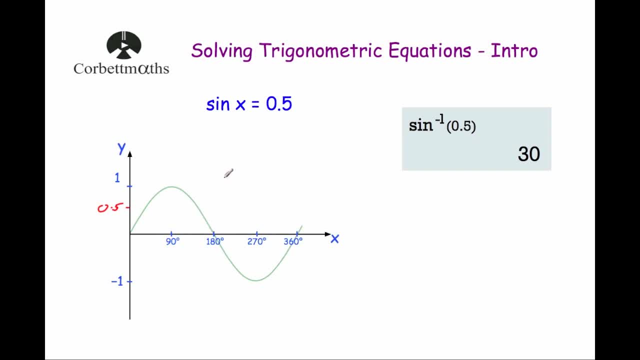 be necessarily one answer. there might be multiple answers and we have to make sure that we get all of them. To do that, we're going to use a thing called the Cast Diagram, So we're going to start off by looking at this diagram here. okay, and this forms the. 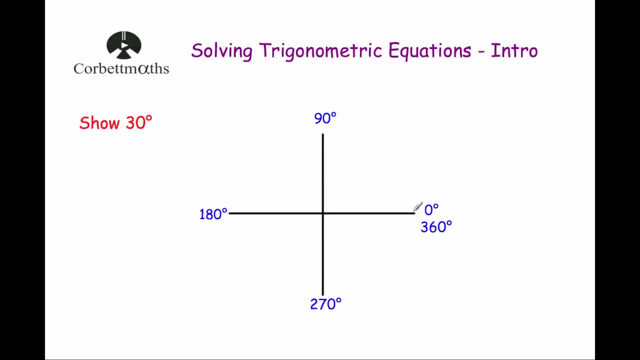 basis of the Cast Diagram. We've got our four quadrants. so we're starting off here at zero degrees And if we go around anticlockwise, 90 degrees. we've got our four quadrants. So it would be here 180 degrees, 270 degrees and back around to 360.. And if you actually 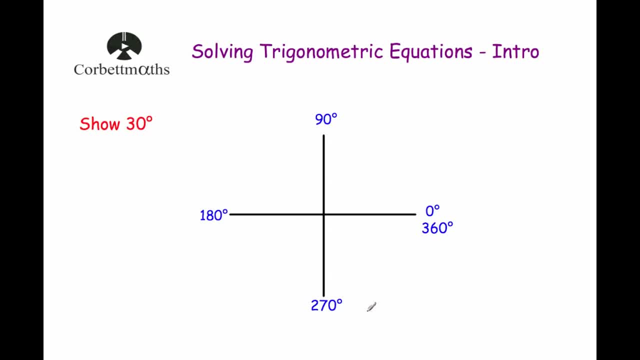 wanted to carry on. we could go to 450 degrees, 540 and so on, So you could just keep on going around. You can also have negative degrees, so you have negative angles, so that would be going around clockwise, and we'll talk about that in another video. Okay, so first of all, 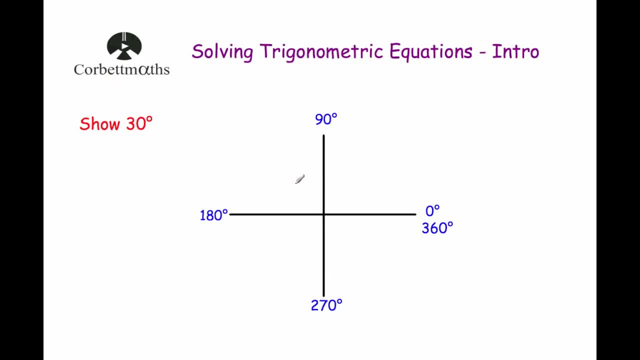 we're going to look at how to show an angle on this Cast Diagram. So let's show the angle 30 degrees, So we've got zero here. we're going to go around to 30 degrees, So a 30 degree angle would look something like this: 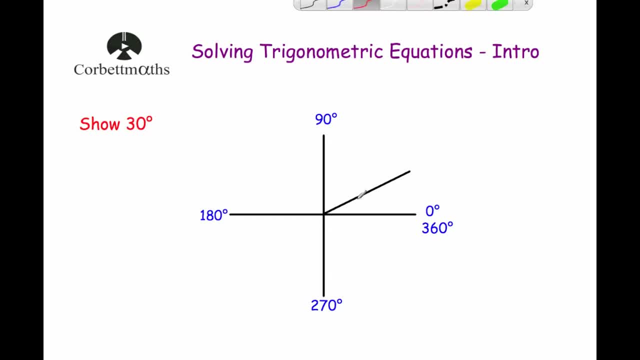 We would go up to here and the angle in there would be 30 degrees, And the angles are always measured from this line here, from where the zero is here. Okay, so the beginning of the first quadrant here. Okay, so we go around, that's 30 degrees. Our next question is to 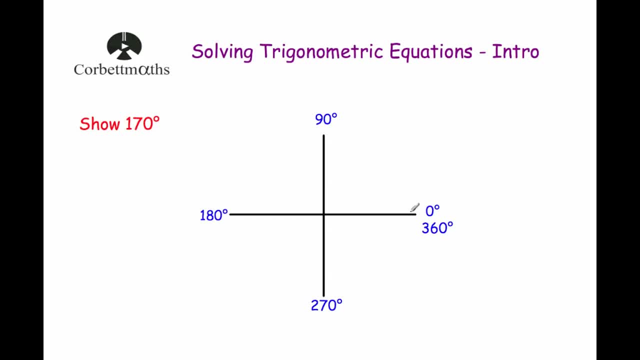 show 170 degrees on the Cast Diagram. So 170 degrees, we would start at zero. we go around to here, to where 170 degrees, So 170 degrees as a sketch would look something like that: So 170 degrees. And our next question is to show 300 degrees on the Cast Diagram. So we're 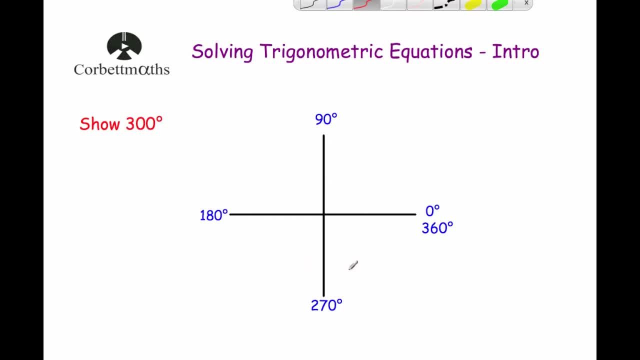 going to start at zero. we're going to go around to 300 degrees, So it would be 30 degrees beyond the 270, so around about there. Remember, these are just sketches And we will mark in our 300 degree angle like so: And that is the angle shown on the diagram. Okay now. 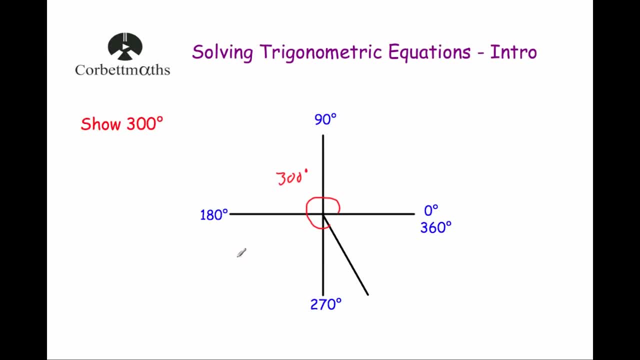 let's have a look and see why the Cast Diagram is called the Cast Diagram and how it's useful in solving trig equations. So let's first of all look at the y cosine x graph. So here we've got the y cosine x graph. 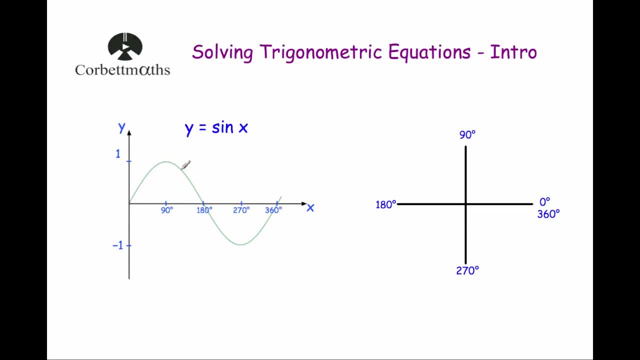 starting at zero, zero going up to one at 90 degrees. zero at 180 degrees, negative one at 270 degrees, zero at 360, and so on. I'll just repeat, And let's have a look at each of the, let's have a look at the values of y for each value of x. So for our angles, 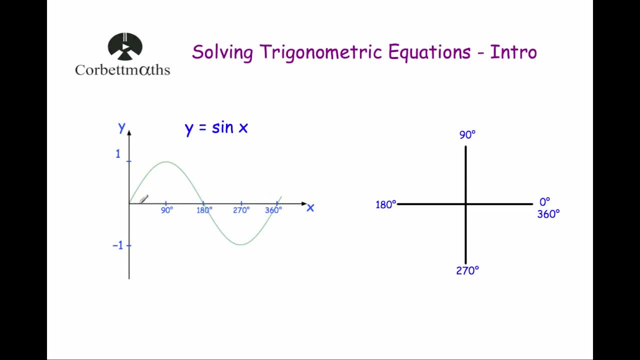 between zero and 90 degrees. so our acute angles, so our, you know, going from zero to 90, our acute angles. As you can see, whenever we work out the sine of those angles, we always get a positive answer. So any of these values between zero and 90 degrees, we will get a. 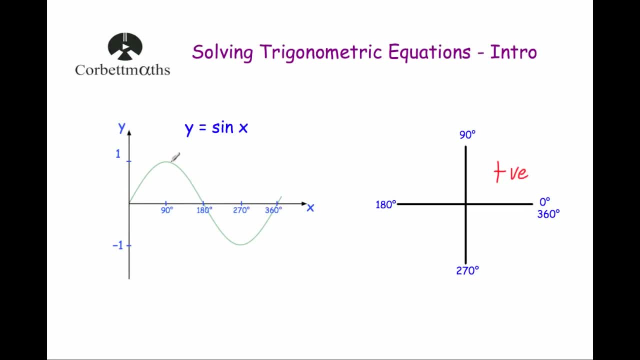 positive answer. So it'll be positive for a sine graph For angles that are between 90 and 180 degrees. so our obtuse angles, they're going to be positive as well, because obviously if you do the sine of 150, you get zero point five and so on. So all those values. 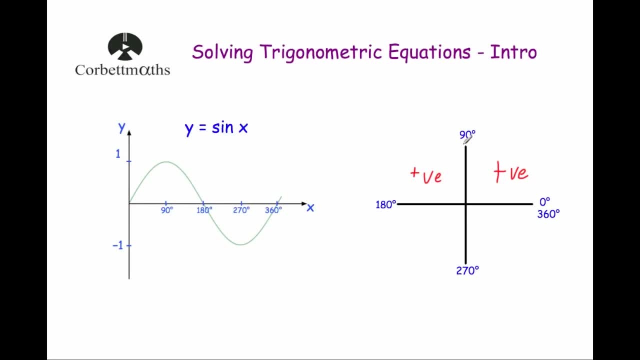 for sine X are positive. So we're going to write positive in this quadrant between 90 and 180 degrees For our reflex angles. well, all reflex angles between 180 and 360, so 360 for reflex angles. between those values, They're all going to be negative. So they're going to be negative here. 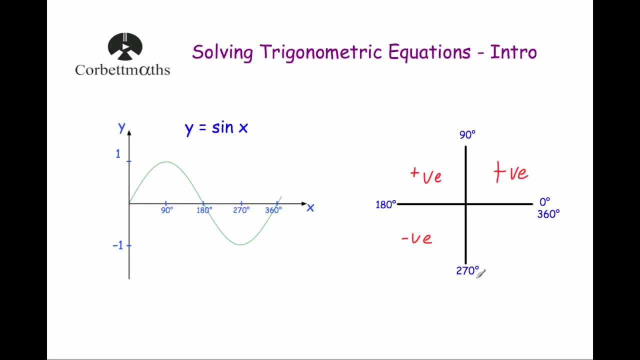 So angles between 180 degrees and 270 and angles between 270 and 360, and negative as well. So for the y equals sine X, or for sine X Our angles between 0 to 90 were positive. between 90 and 180 are positive. 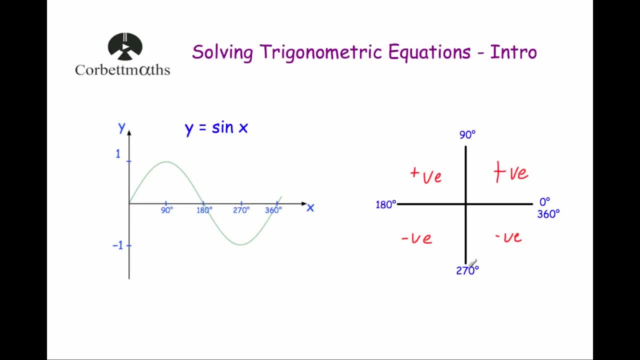 sine of angles between 180 and 270 are negative and between 270 and 360 are negative. Let's have a look now at the cos graph. So y equals cos X between our acute angles between 0 and 90 degrees. Well, they're positive, So they're positive. 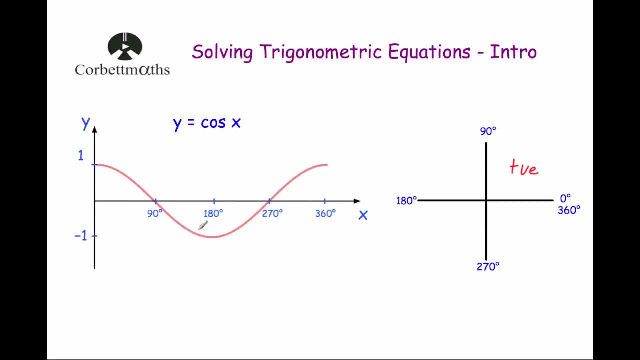 Between 90 and 180 degrees, Well, they're going to be negative. Between 180 and 270, they're negative. and for angles between 270 and 360, The cos of those angles will be positive. Okay, and finally, the time graph. if we 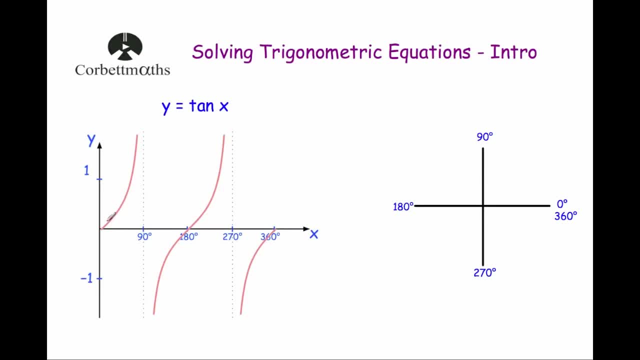 Look at the time: graph y equals tan X. if we work out the tan of angles between 0 to 90, Obviously 90 is an asymptote, But if we do the tan of angles between 0 to 90, they're going to be positive and 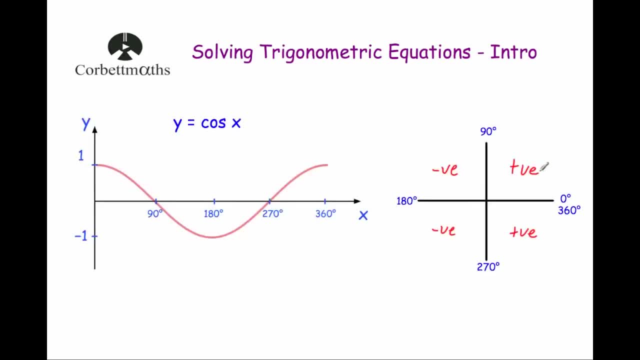 If you notice, all first quadrant angles are positive whenever you work out the sine, the cos or the tan of them. angles between 90 and 180 degrees are negative for tan, between 180 and 270 are positive for tan and between 270 and 360 they are negative for tan. 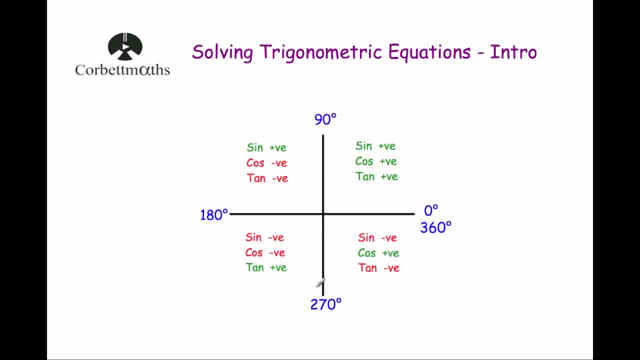 So what we're gonna do is we're going to have a look at that, So put that into one diagram. the sign, the cause and the term were all positive between naught and ninety degrees. So that quadrant we're gonna call a. in this quadrant, So angles between 90 and 180 degrees, when we work out the sign, the cause and the town, of those angles only the sine. 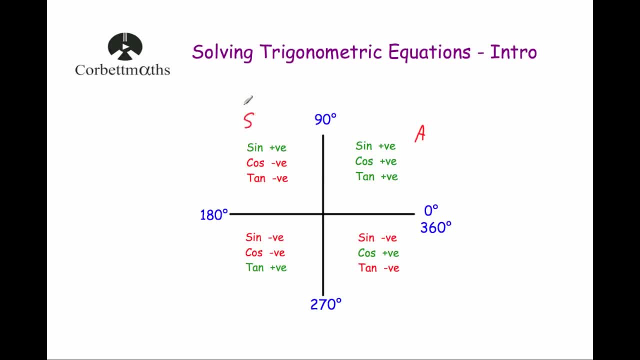 Of those angles are positive. So in this quadrant we'll call that quotient s angles between 180 degrees degrees and 270 degrees. when you work out the sign, the cause and the time of those angles, only the time of those angles will be positive. so we're going. 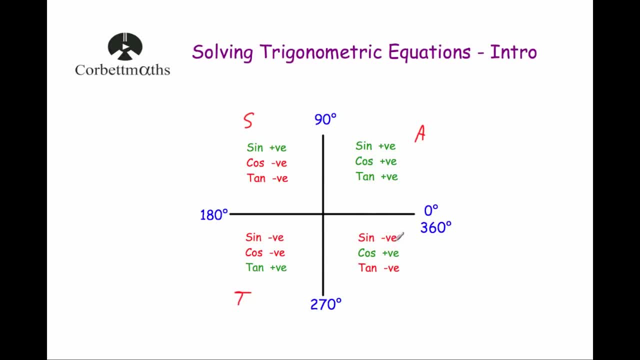 to call this quadrant T and this last quadrant here. whenever, for angles between 270 and 360, whenever you work out the sign, the cause and the time of those angles, only the cause of those angles are positive. so we're going to call that quadrant C. so there, we've got our C A S T and that is your cast. 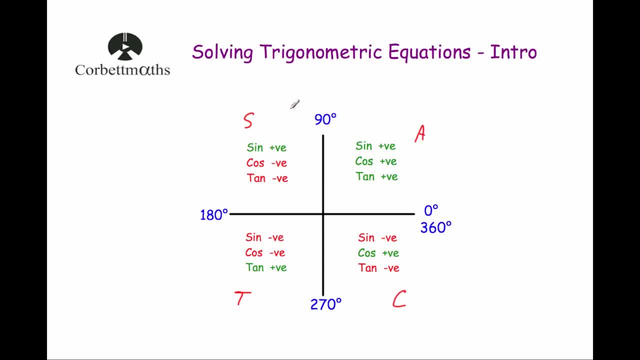 diagram. just remember that the A goes into the first quadrant, so A, S, T and the C there. okay, so that's the cast diagram now. it's really useful for working out or helping you solve trig equations, and let's have a look and see why. now let's 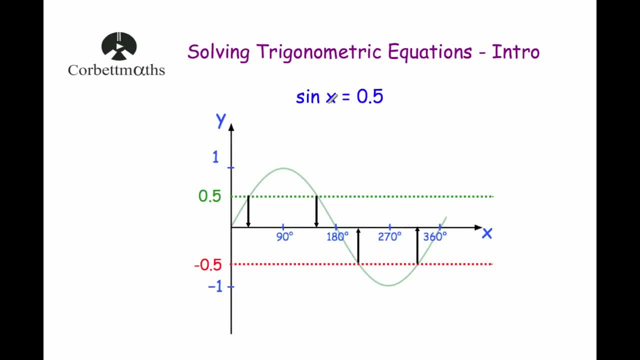 have a look at that first question. we started the video with sine X equals 0.5 and we're gonna have a look and see why or how the cast diagram will be useful in solving that question. so, as you can see, we've got the sine graph here and 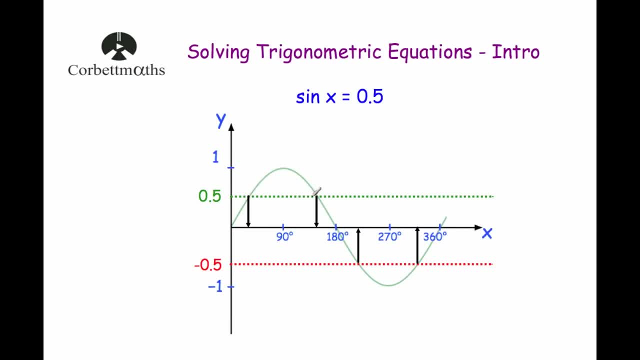 what I've done is I've shown where the graph equals 0.5 and also minus 0.5 or negative 0.5, because that's going to be quite useful. so I'm going to show you how to do that and I'm going to show you how to. 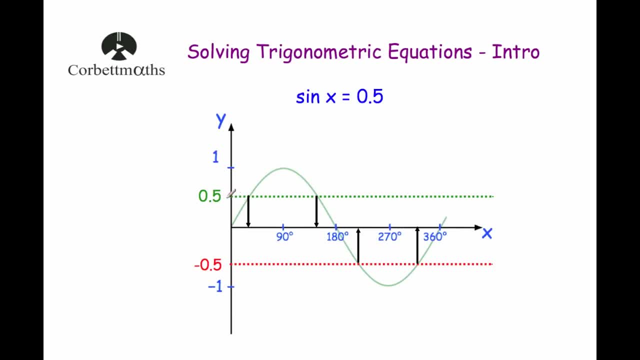 use for whenever, using the cast diagram also. so we've got here. obviously we know the sine of 30 is 0.5, so 30 degrees would be one of the angles. now the next one would be 150 degrees, because if you take 30 away from 80 you will get back. 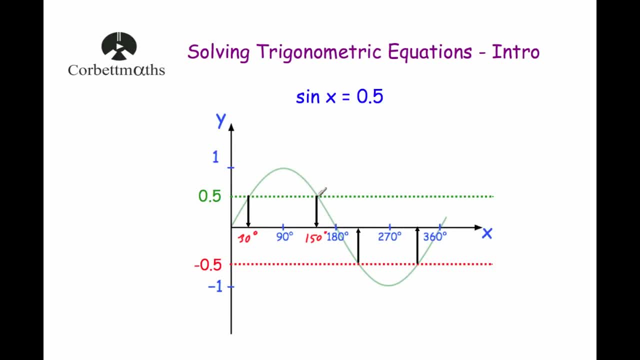 to the over location where the sine X is equal to 0.5. so whatever that angle is at 30, if you take it away from 180 you'll get the over value there on the sine graph. now, interesting, I'm just going to identify where these two angles are as well. where sine X. 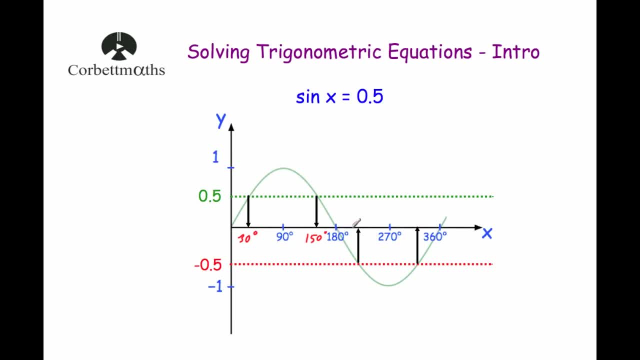 is equal to negative 0.5. so this one, it's another 30 degrees past 180. so that would be 210 degrees and this angle here would be 30 before 360. so if we take 30 away from that, we'll get 330 degrees. now, obviously, the answers to this question. 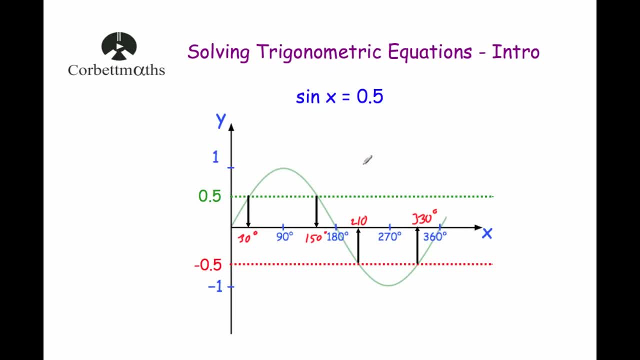 would be if we were asked to solve this question for angles between naught and 360 degrees. our answers would be 30 degrees and 150 degrees. but I've just shown the negative angles on the diagram just to show you how that sort of links in with the cast diagram. so, as you can see, here we've got the negative angle. 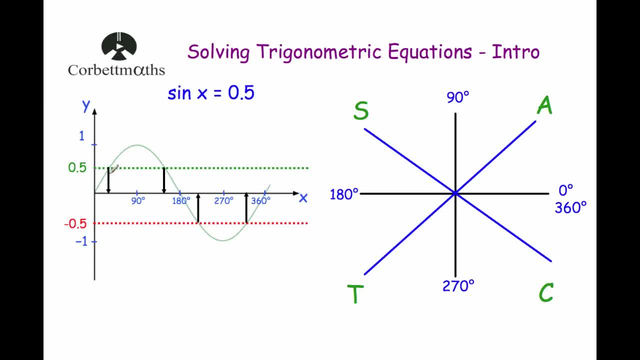 here and we've got our first angle. our first solution was 30 degrees, so let's just have a look at that on the cast diagram. so our first angle here is equal to 30 degrees and that is one of our solutions. and we know that because 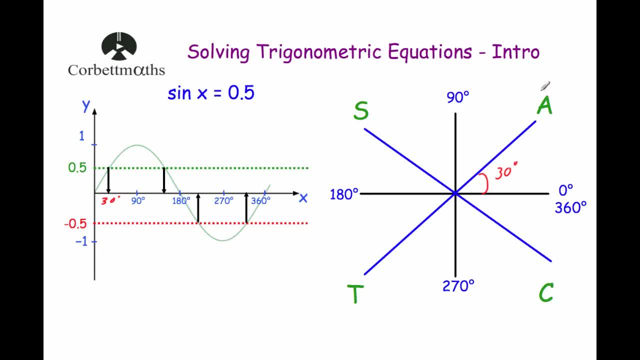 we're looking for. whenever sine X is 0.5, that's positive and a all a positive in this quadrant. so that would be one of our solutions. our next angle? well, our next angle is this angle here, which is 150 degrees. I'm actually sure by just 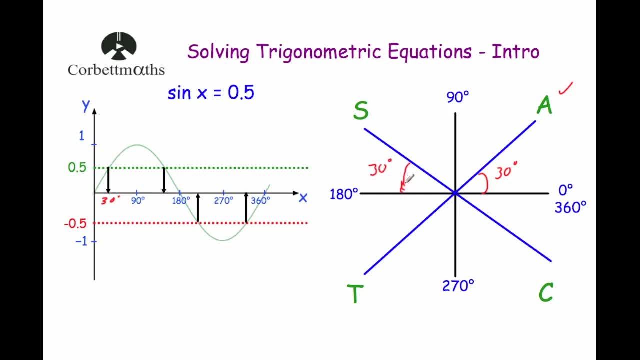 putting a 30 degrees in here, because I know that it's 30 degrees before 360 degrees before 180 degrees, so that's going to be 150 degrees and again the it's s. that means the sign is positive. so, yeah, that's one of our solutions. our next: 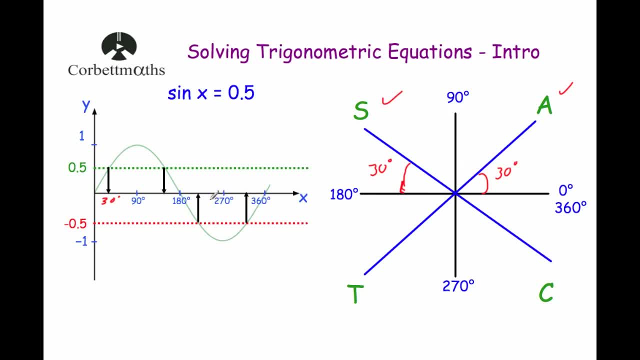 angle- and this wasn't a solution, but I'm just going to show it because it was a key one- on our diagram was 210 and I just show that by putting in over 30 degrees there and that's 210. if we start from 0: 210 degrees and now only the. 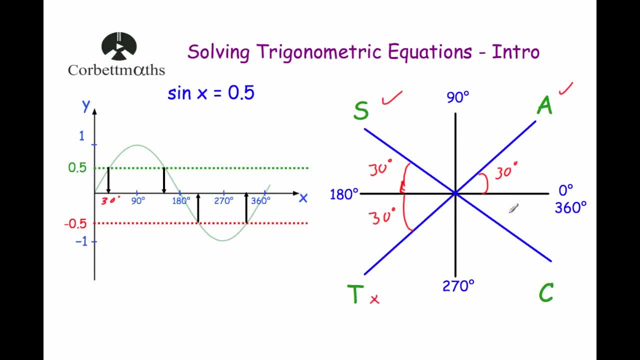 tans positive in that quadrant. so that's not one of our solutions. and our last angle of interest is this one: our negative 0.5. the sine of 330 is equal to negative 0.5, so I'm just going to put 30. 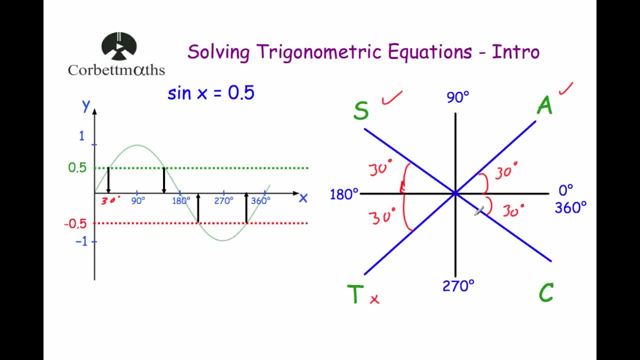 degrees there, because 330 degrees would be that angle there. but that wasn't one of our solutions because we wanted to find whenever sine X was positive 0.5, and that's it. so this cast diagram can be very useful in solving these trig equations. let's have a look at a question now and see how we can use it. 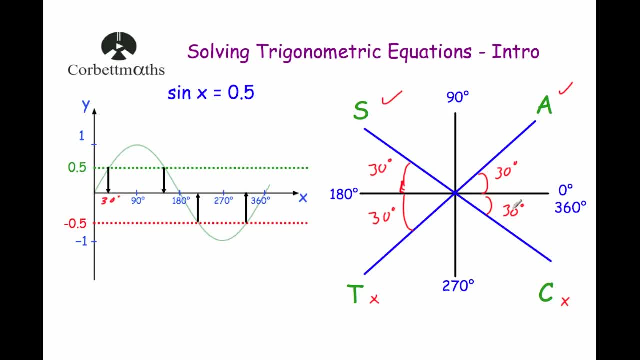 without having to draw the trig graph, and this could be particularly useful because if we were asked to find it between 0 and 720 degrees, we could just go around the diagram again. okay, so let's have a look at our next question. so our next question is to solve: tan: X equals 1, so what I'm going to do is I'm 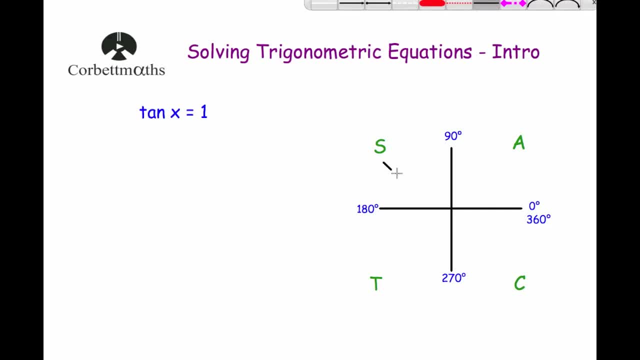 going to draw the angles on the angles of interest onto the cast diagram straight away. okay, so I'm going to put in the lines like so, rather than draw the time graph, and what I'm going to do is I'm going to find this first angle here, and to find this first angle, we're just going to do the inverse tan or the. 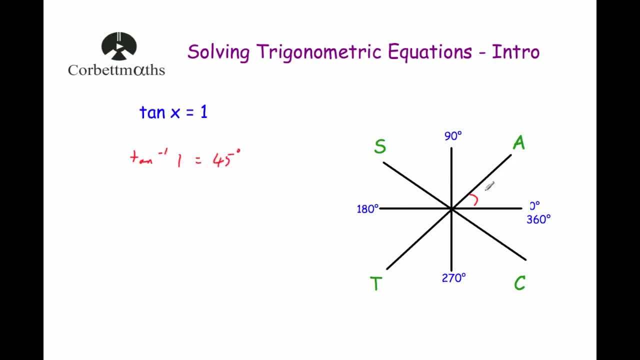 arc tan of 1 and that is equal to 45 degrees. so this angle is 45 degrees over our angles of interest. then would be this angle here 45 if we put that in, which would be 135 degrees, it's 45 degrees before 180. this angle here which 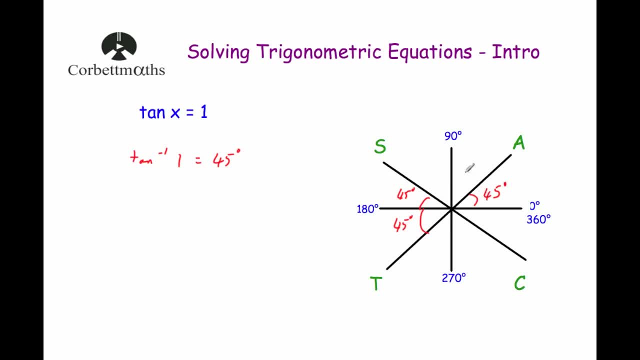 is 45 degrees, after 180, which would be 225 degrees, and this angle here, which is 45, in there, which would be 315 degrees. so they're all angles which would be either 1 or negative 1 whenever you work out the tan of them, okay, so 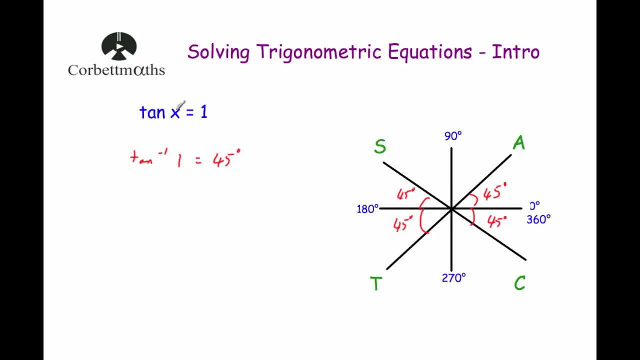 we want to find the angles which we give. whenever we do the tan of it, we should give positive 1. so let's have a look at our cast diagram. so in our first quadrant all of the angles are positive. so tan is positive here. if you do the. 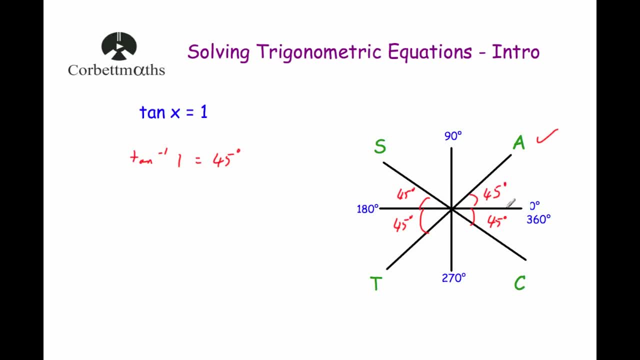 tan of 45 degrees, you get a positive answer. so our first answer will be 45 degrees. so that's our first answer. X equals 45 degrees. or, if we carry on round and this quadrant, only the sign is positive, where we're wanting an answer of 1, which is positive, but only signs positive, so that wouldn't. 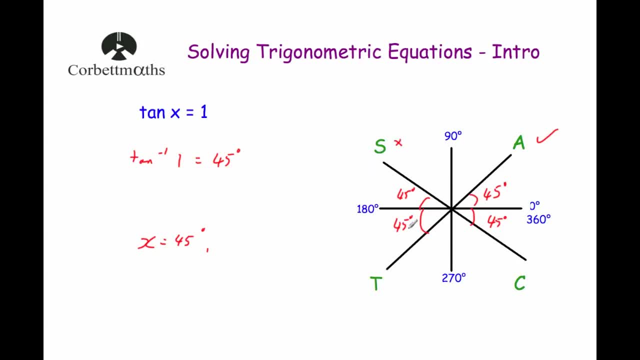 give us a solution if we carry on round this one, this quadrant. the third quadrant, tan, is positive, so that will give us a solution here. so we want to find what this angle is. so we're going to start from zero and we're going to go round to 180 and then add on another 45 would be 225. so our next- 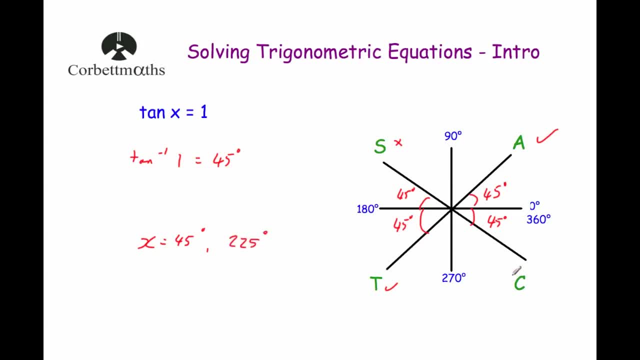 solution would be 225 degrees. and then our last quadrant. I always check: only the cause is positive here. obviously this is tan, so that won't give us a solution, and that's it. so if we wanted to find the solutions or the angles to tan- X equals 1- our values for X would be 45 degrees or 225 degrees. so the cast. 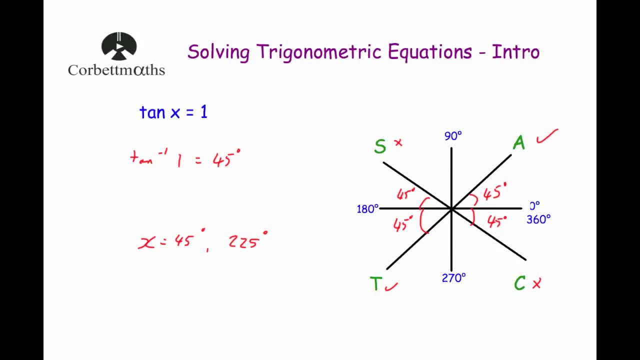 diagram has just given us a way to solve that really quickly and simply without having a look at the graphs. if we do look at the graphs, as you can see, our values of 1 would be here at 45 degrees. our next one would be over here at 225. 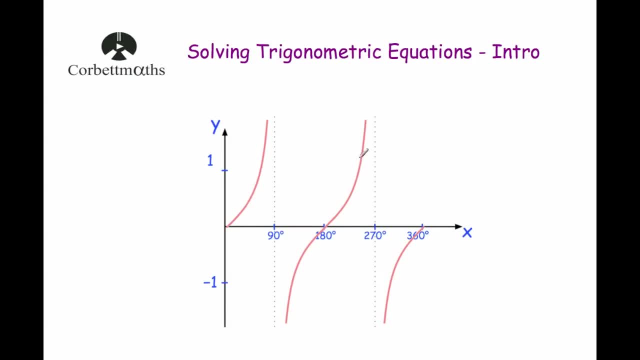 degrees. so you can sort of check with the diagram if you, if you want to. but as you use the cast diagram over and, over and over again, you can just solve the equations, the trig equations, so quickly and simply. okay. now last question is to solve. cos X equals 0.9 and we'll solve it. 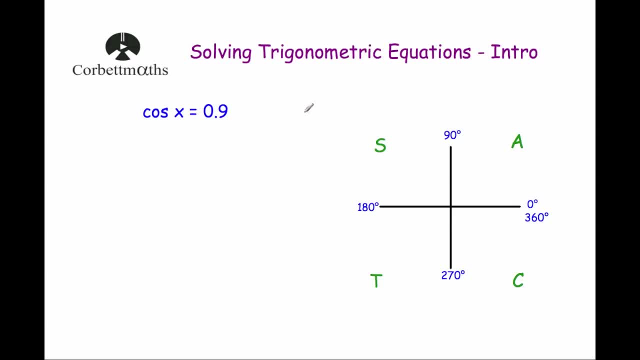 for angles between 0 and 360 degrees. so first of all, what I'm gonna do is I'm gonna work out the arc cause or the inverse cos of 0.9, so that will tell us the angle, obviously in the first quadrant. so whenever we do that, we get 25.84, and so 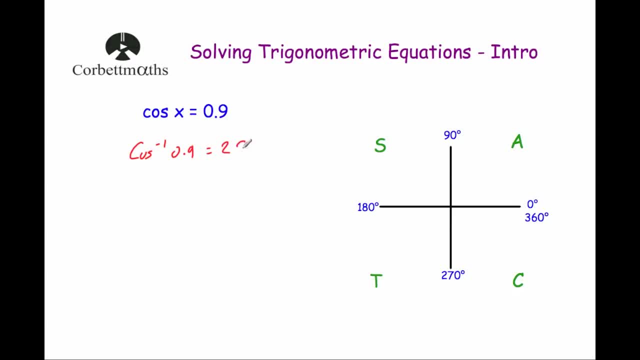 on. I'm just gonna use it to one decimal place in this question. so I'm gonna go for 25.8 degrees and what we're gonna do is we're gonna mark that on the cast diagram. so let's mark that in for all the quadrants: the angle of 25.8. okay, so obviously. 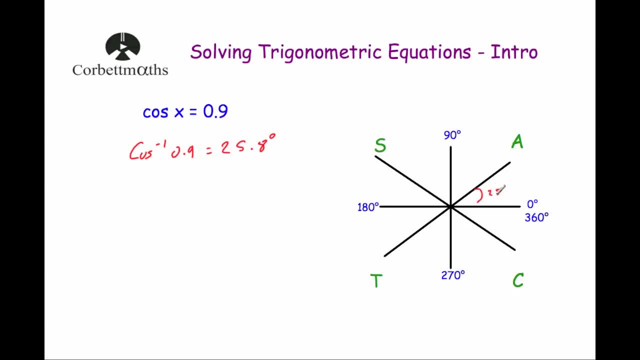 we want the first angle of 25.8 degrees. the next one, obviously it's going to be 25.8 degrees before 180 degrees, 25.8 degrees after 180 degrees and 25.8 degrees before 360, and they will be the. 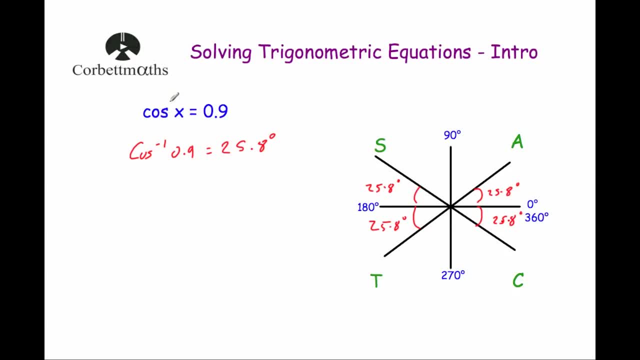 angles that are either 0.9 or negative- 0.9- and whenever we work out the cause of that angle or those angles. okay, so we want to find that whenever it's positive. so obviously it's 0.9, so it's positive. so if you have a look here, let's take the quadrants, which would be a give us a positive answer whenever.